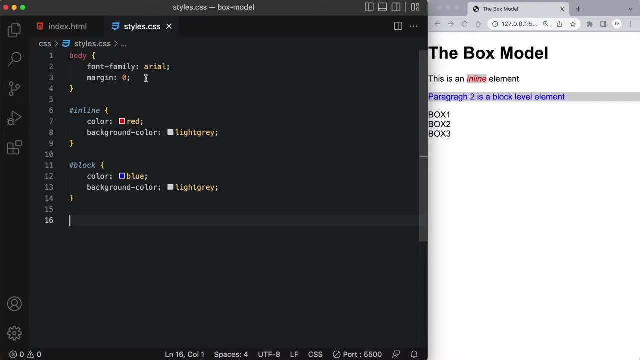 Arial just to change the text styling and a margin of zero to remove any default margins that the browser may have provided. Now I've targeted my ID of inline and block and applied some styling to them. Now inline is targeting this m-tag that I have here with the text inline: 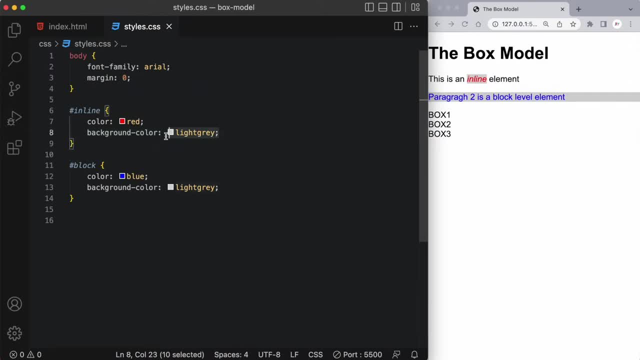 within it. I've given the inline ID a background color of light gray and you can see it only takes up this little bit of space. So I've given the inline ID a background color of light gray and that's because an inline element only takes up as much width as necessary. so as much width as 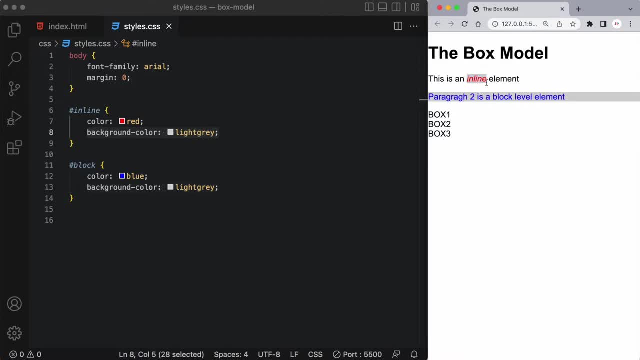 its content And it doesn't start on a new line and it doesn't push any content after it onto a new line. Now, because this is a new paragraph tag, this is starting on a new line And what I've done here is I've given it a background color of light gray to demonstrate that, because it's a 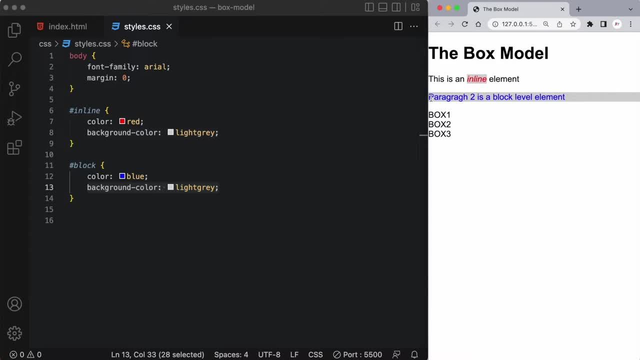 block level element. it's going to take up the full width that's available to this element. So what I've done here is I have these three divs with IDs of one, two and three respectively and the text box one, two and three within them, And you can see these three boxes here in the 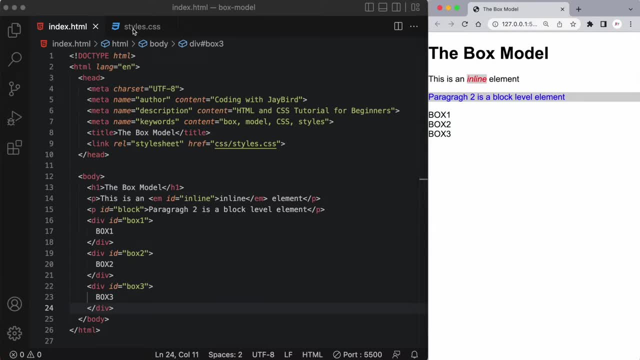 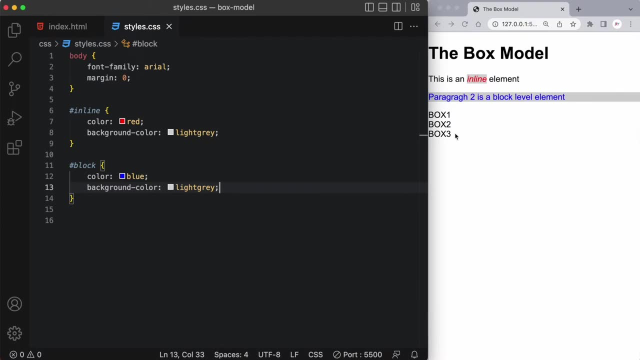 browser on the right, So I'm going to use these three to demonstrate what the box model is and how it works. By default, the browser looks at every element on our web page as having a box around it, So each box is going to take up the width of its content. Now the content is really. 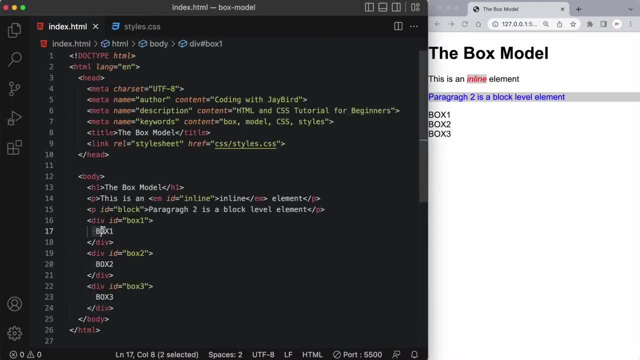 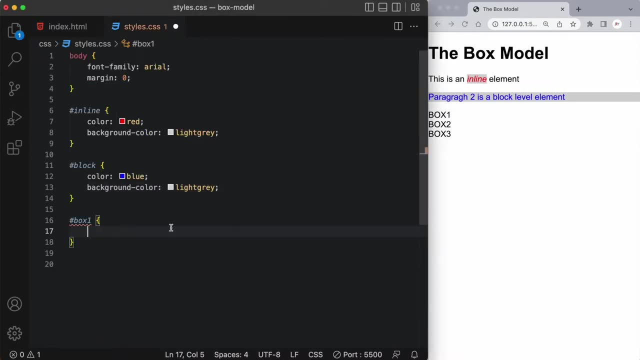 just the text and the images that it's going to take up. So I'm going to use the box model here to demonstrate what the box model is going to take up. So in our case, our first box has the text box one within it. So that's the content and that's what we see here. So what I want to do is I want 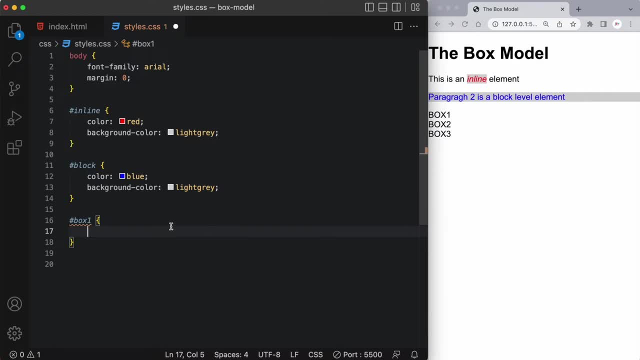 to demonstrate a few concepts such as padding, margin and border. So what are they? Well, we already know that the content of the box is the text box one. Now, if I were to add a background color, let's say of light blue, we'd see that the div takes up the entire content of the box. So 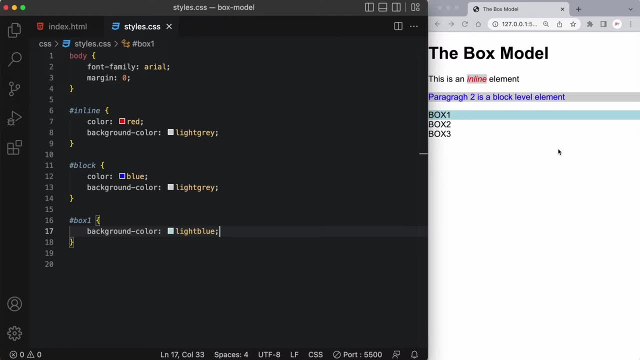 if I were to add some padding to this box, we'd see that we'd have more light blue surface area around the word box one. So let's add a padding of, let's say, 20 pixels And we can see. now we've. 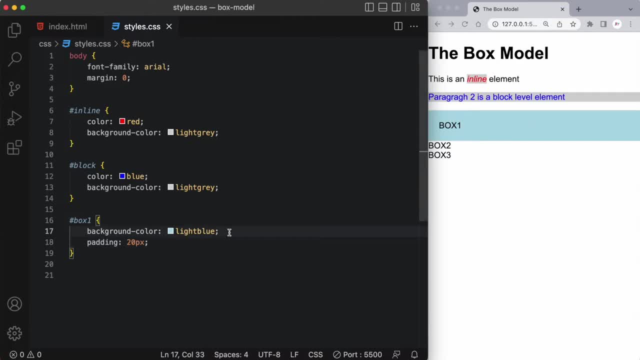 increased this area around box one. Now, if I were to comment on this box, I would say: out this background color. we'd see that there's no color around this, And that's because padding by default is transparent. So only when you have a background color applied to it can you see the 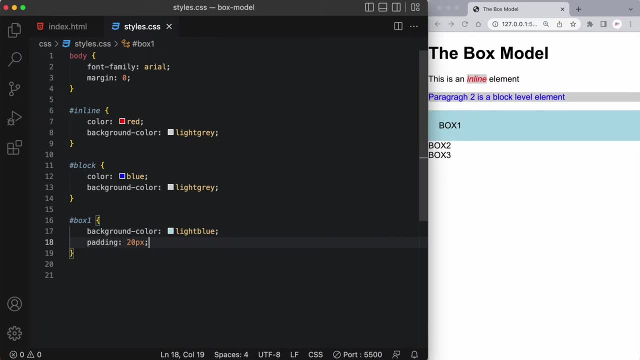 padding in itself. Next, I want to talk about the border aspect of a box model. Now, the border wraps around the content and the padding of a particular element. So if I were to create a border here in box one, it's going to wrap around all the blue that we see here in our browser, So I can write. border here in box one. And if I were to create a border here in box one, it's going to wrap around all the blue that we see here in our browser. So if I were to create a border here in box one, it's. 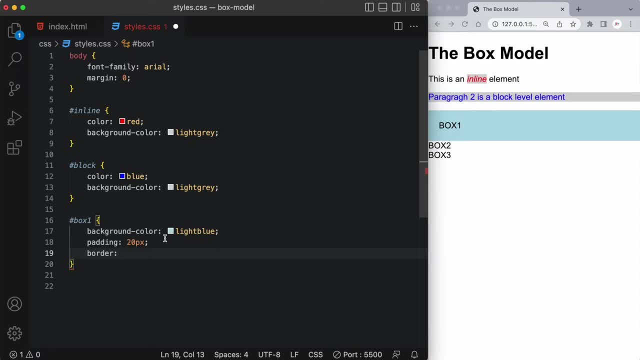 going to wrap around all the blue that we see here in our browser. So if I were to create a border in three separate lines where I can give it like style or color or sizing, or I can have a short form where I put all three in one line, which I'll do here. So I'll say five pixels and I want the 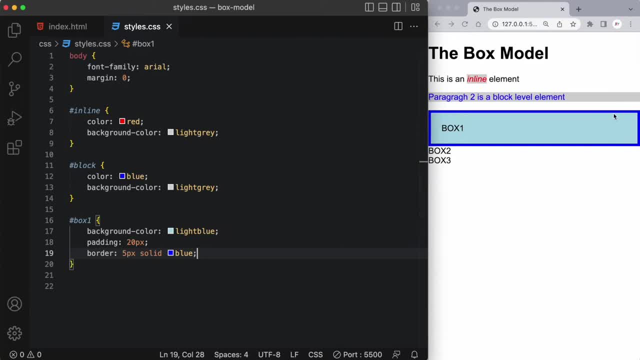 line to be solid and the color blue, And you can see. we've created this border around box one, which is the content as well as the blue padding within it. Now, in order to better understand the box model, I'm going to give each one of these divs a height and width to make them look like a box. 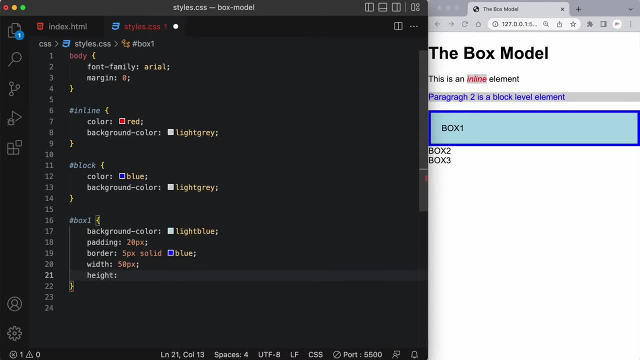 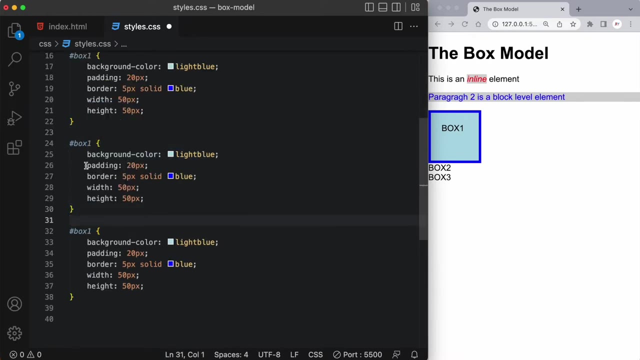 So I'll give this a width of 50 pixels as well as a height of 50 pixels. Now I want to take this styling and replicate this once again in box two and box three. So I'm just going to copy this two more times And then what I'll do is I'll actually change the styles to have slightly different. 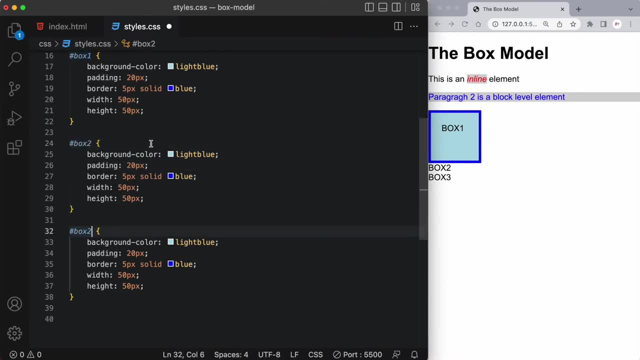 colors so we can see the difference. So I'm just going to say box two and box three. maybe the second one will be light pink And I'll give it a color for the border of red. And then I'm going to give it a color for the last box And we'll give it a border color of green. Oops, what have I done? 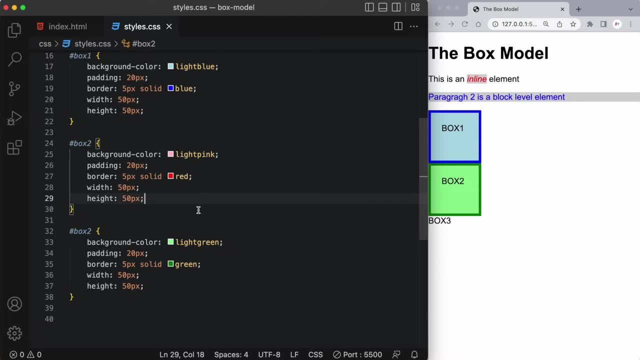 wrong. That's not what I expected. Let's ask my handy debugging duck, Tim, to see what's going on. Hmm. so what have I done wrong? Everything looks good, Not missing any semicolons. Ah, I've written box two twice for the IDs, So I'm actually overriding this. 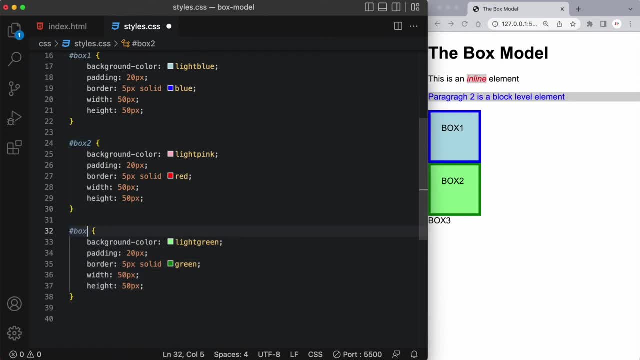 These styles with these styles. So let's change this box two to box three, And now that's what I expect it to look like, where we have a blue box, a red box and a green box. Now you can see, these boxes are stuck together. Now the way to create space between these boxes would be to add what's. 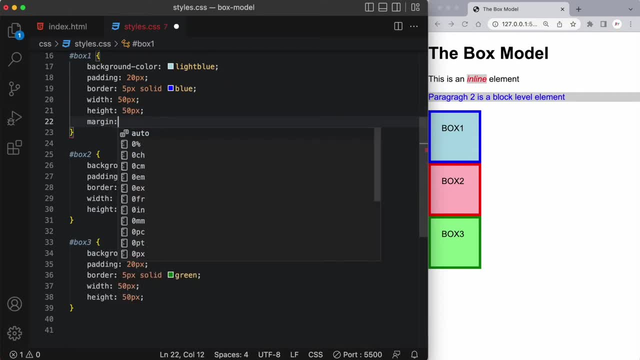 called margin. So let's go ahead and add margin to our first box of 60 pixels. Now, what margin does mean is always transparent as well, similar to padding. So when I save it, we're going to see that we've pushed this blue box 60 pixels away from the left side of the web browser and 60 pixels from 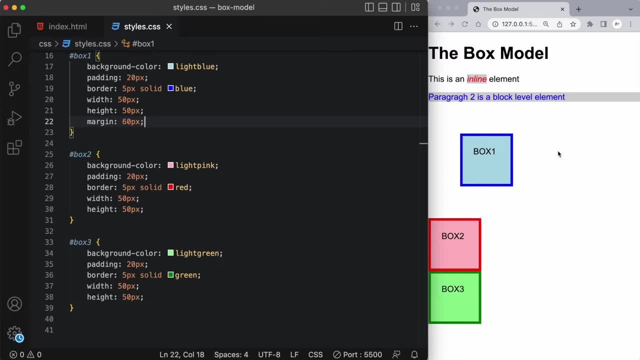 the top element and then 60 pixels from the right- But the right has tons of space so we don't really see it- and 60 pixels away from the box below it. So the way I like to look at the box model is this: 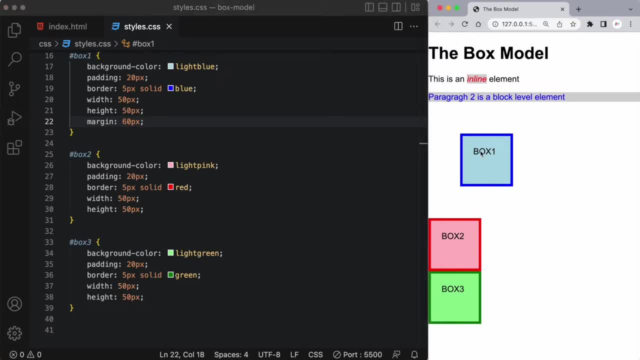 I like to think of myself or a person as the content itself. So let's say the text box one is a person. Now, this person box one is wearing a jacket. So let's say, the outer shell of the jacket is this border that you see here. 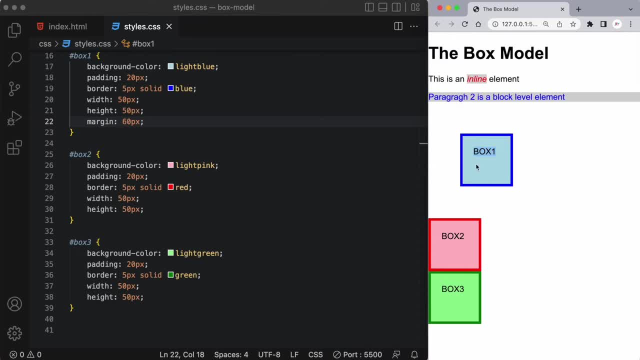 and the stuff inside of it. So this blue background color or the padding is kind of like the padding or like the filling of the jacket. So let's say you're wearing a winter coat and it's full of down. that winter jacket would be full of the padding or the down, So the person is wrapped with some. 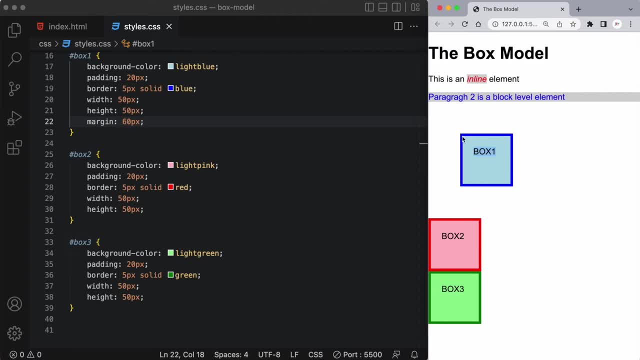 down padding. then they have this border, which is a shell of the jacket, which can have some thickness or different styling based on the kind of jacket you're wearing. And now imagine this person is standing in line with other people. So these are the other two people: the red box and the green box. 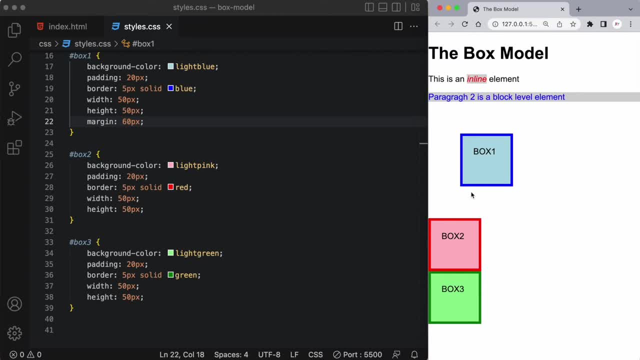 So when this person wants to push themselves away or create a space between them and the next person in line- So let's say you're wearing a jacket and you're wearing a jacket and you're wearing a padding- So let's say they're social distancing and they just want some distance between them. 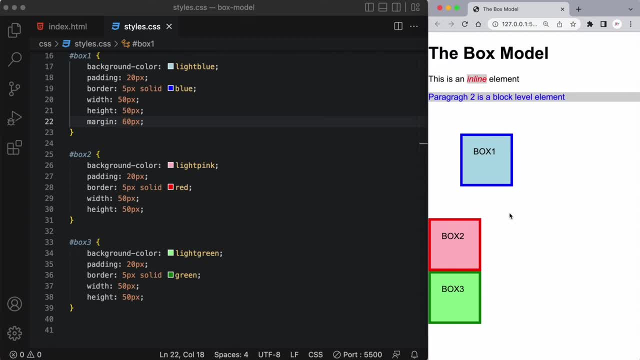 and the next person. they're going to add margin, So margin creates space between this person who's wearing this jacket with some padding, and it pushes them away from another person somewhere else on the web page. Let's have a look at this in the browser dev tools. So using my select tool. 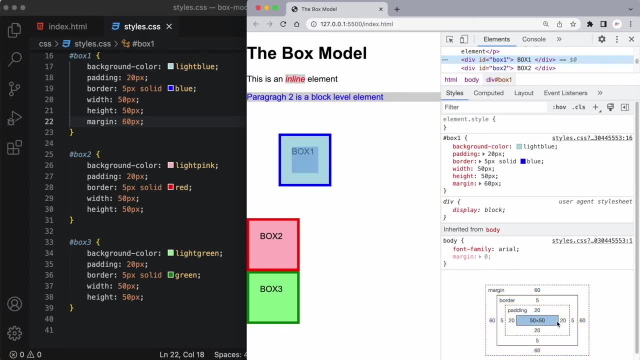 I can select the first box and I can see this area showing up with padding, border And margin. So if I hover over the inside here, where it says 50 by 50, that is the width and height of the box that I've set. So that's the content itself. And when I hover over the padding, 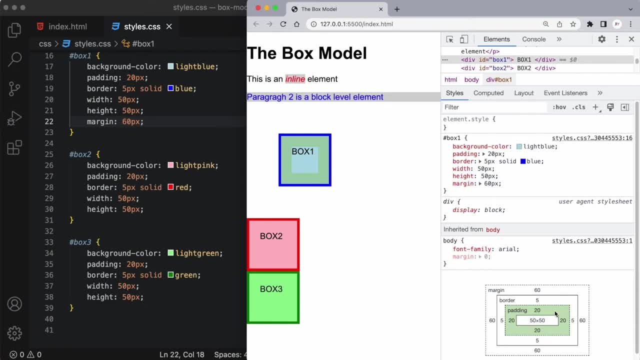 you can see that it's highlighting the area around the content box, one in the web browser. So that's like the filling of my jacket. And if I hover over the border, you can see that now it's highlighting the blue border around this padding and content. And now, if I hover over my content box, 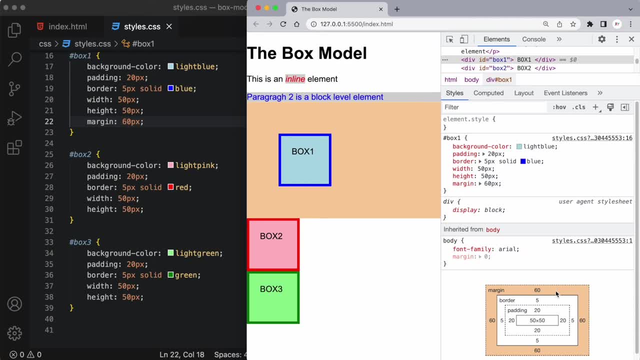 margin. you're going to see all this extra space that I've created outside of my border content and padding, and what that's doing is it's pushing the other elements away. All right, so let's demonstrate a few more things in our second and third box. I'd like to give my second box a margin. 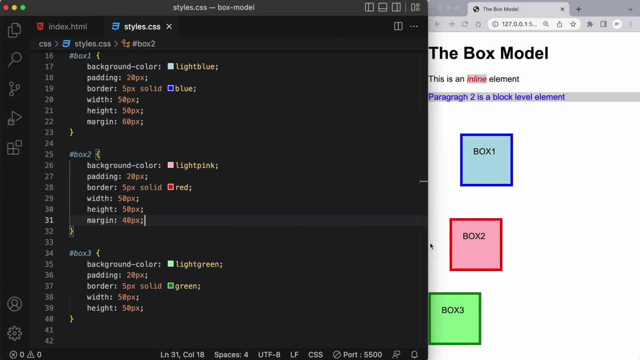 of 40 pixels, and now you can see it's pushed away from the left browser wall a little less than this one, and that's because this has a width of 60 and this had a width of only 40 pixels, and it's also adds a margin to our third box, so I'll add an even smaller amount of, let's say, 20 pixels. 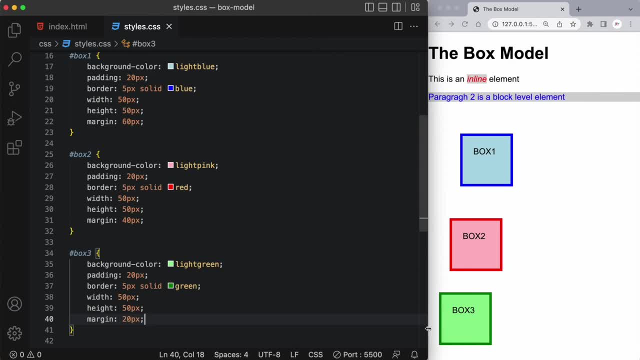 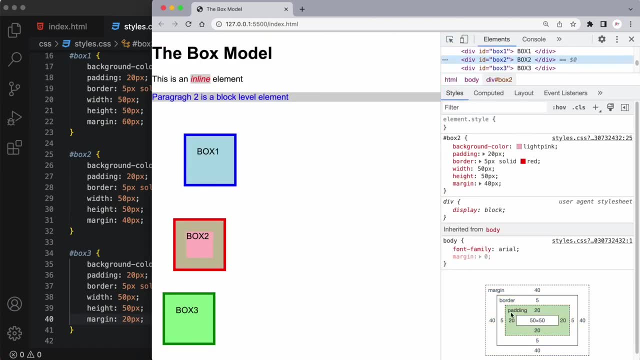 and we can see it's even closer to our left wall of the browser. Now let's open up our dev tools to have a better look at this. So here, if I select my second box, we can see we have margin of 40.. Now the margin of 40 is taking up the entire distance between box 2 and 3 in here. and why is? 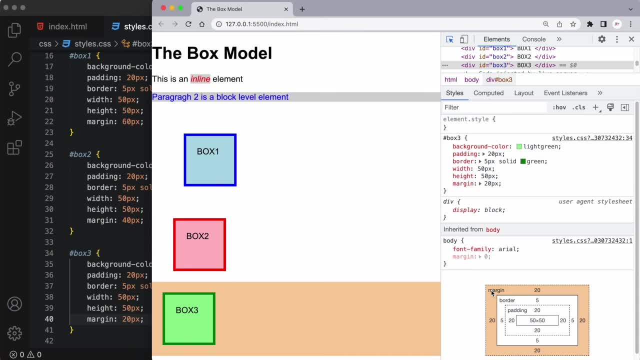 that If I target the third box, we can see its margin is coming up as 20.. And it's not taking up the full space between box 2 and 3.. So why is it that box 2's margin is giving the entire space and creating this distance between them, but not box 3's margin, And that's 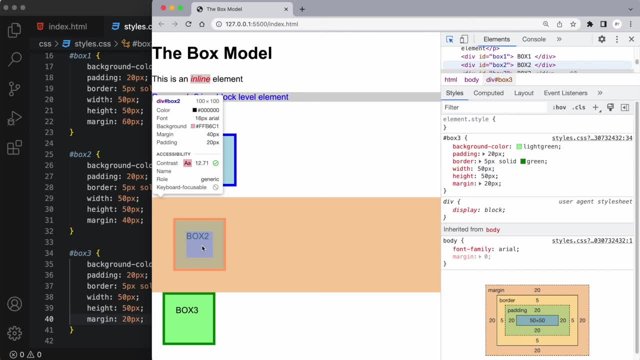 because margins collapse and the larger of the two margins is the dominant value and is the chosen distance between the elements. So box 2 has a margin of 40, so it dominates over the value of box 3's margin, which is 20, forcing this one's margin to collapse. So if I target the third box, I can see the margin of 40 is taking up the entire space between box 2 and 3 in here. and why is that? If I target the third box, I can see the margin of 40, so it dominates over the value of box 3's margin, which is 20, forcing this one's margin to collapse. So if I target the third, 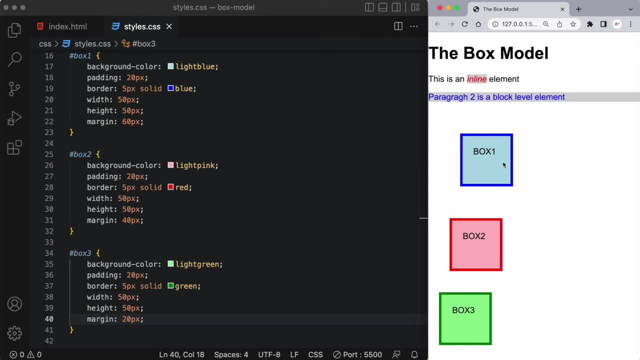 box I can see the margin of 40, so it dominates over the value of box 3's margin to collapse. So if you were to calculate the actual width of an element like, let's say, box 1, you would be adding its width, its padding and its border. So sometimes this makes this a bit. 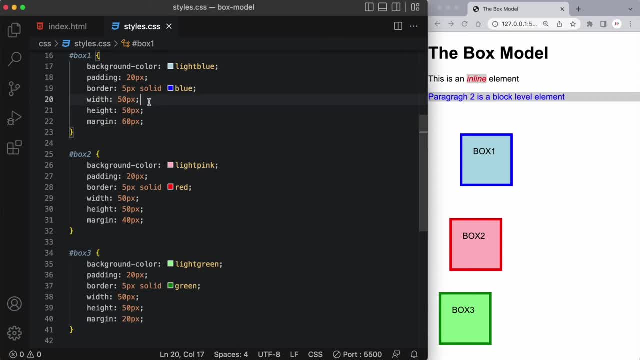 tricky for a web designer, because we think we're setting the width and height of a particular element, but by adding padding and border we end up making this width a lot larger or its height a lot larger, And that's where something called box sizing comes into play. 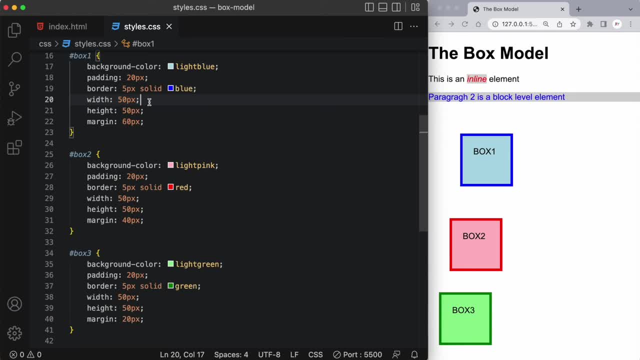 Now, box sizing is a CSS property and it allows us to include the padding and border of the elements: total width and height. So if you were to do that to an element like previous example, let's say I said box sizing property and I give it the value of border box. let's 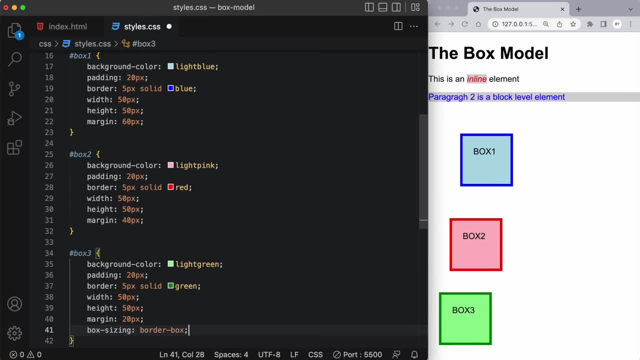 see what it does. box Ok. it makes that box a lot smaller And that's because the box sizing property is allowing us to include the padding and border in that particular elements: total width and height. So now the total width of box three isn't 50. 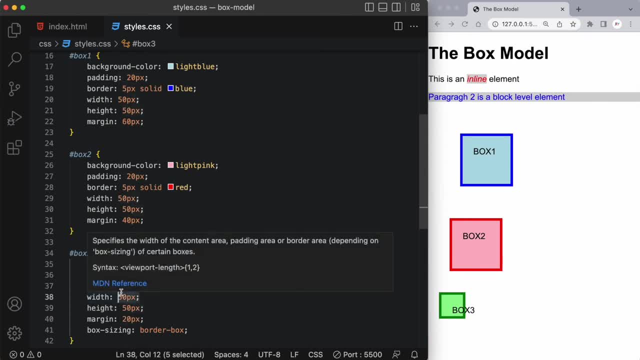 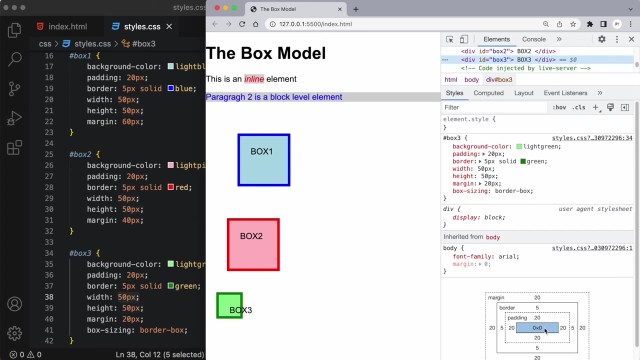 plus 20 plus 5, it's simply 50. And now this padding and this border all has to be squished within that width of 50.. So let's have a look at this in the dev tools. If I target the third box, we can see its content has zero by zero. Okay. 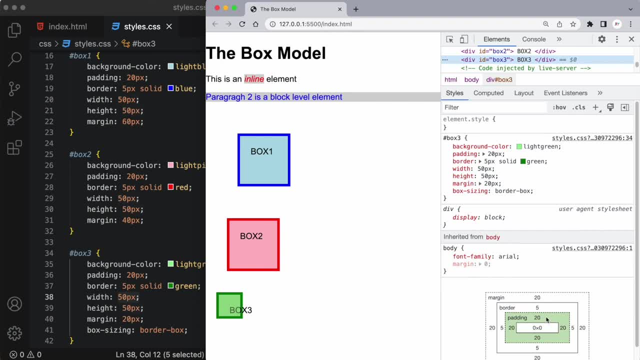 and that's because its content won't fit inside that box. There's the padding of 20 and there's the border of 5.. So if you add the top border, which is 5 plus padding of 20 plus 0, plus another 20 plus 5, you get the total height of 50. 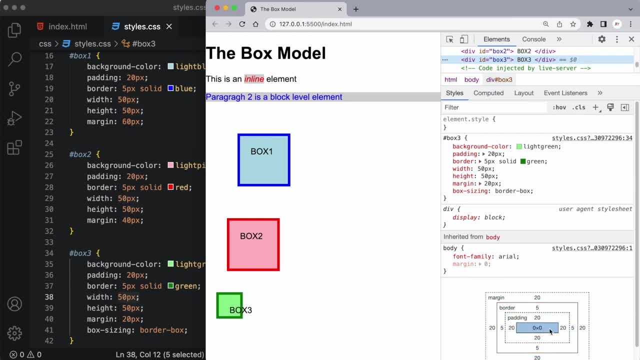 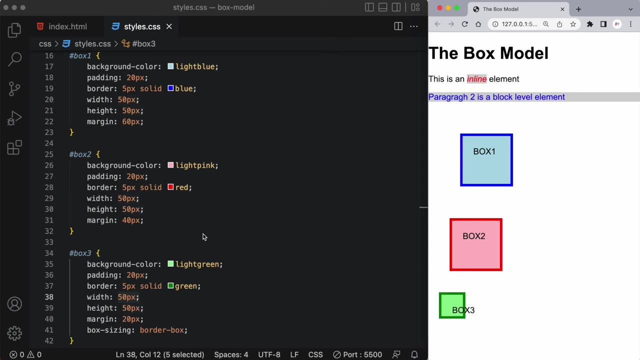 and similarly you get the total width: 5 plus 20 plus 0 plus 20 plus 5 of 50. And then the margin expands outside of this border box sizing, As you can see, applying the property box sizing with the value of border box on. 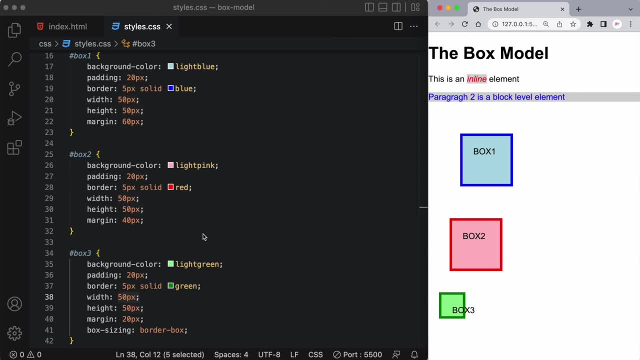 an element is fantastic because it allows us to take the padding and the border and include it in the width and height of a particular element, Just making our design a lot easier to build. Alright, guys, that's it for my video on the box model. I hope you've been enjoying this video so far, If you have.